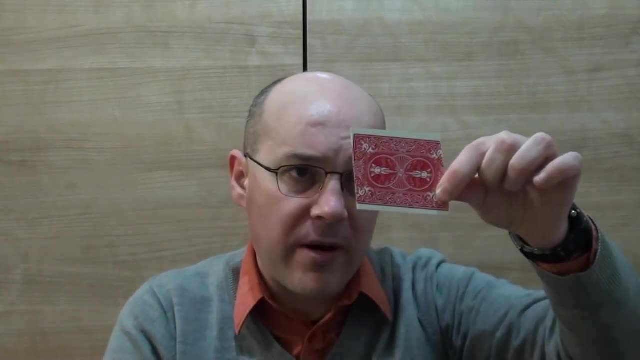 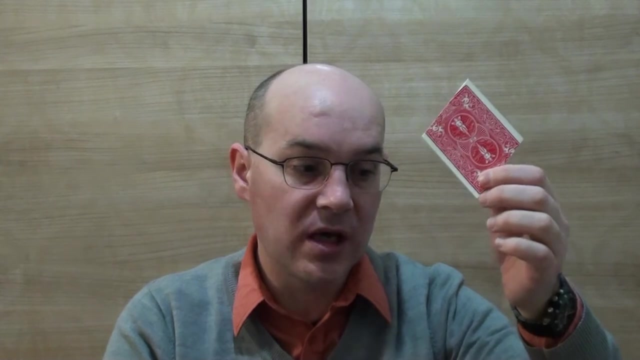 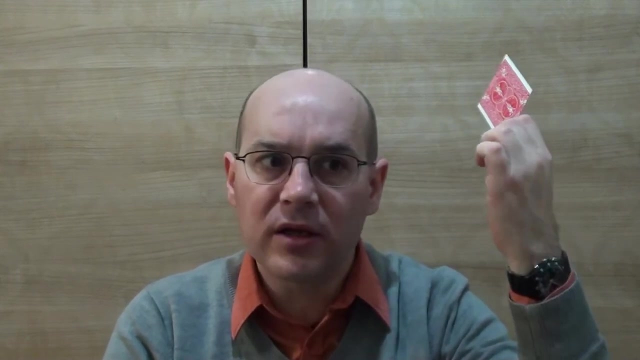 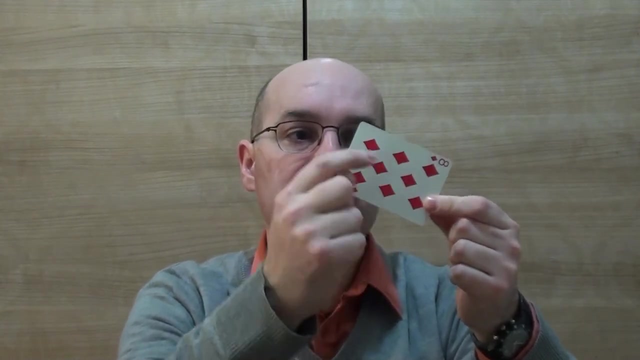 in order to get not just a parallelogram but a beautiful and nice rhombus. So there are two ways to do this, using, of course, rhombuses, symmetry and diagonals properties. So to find your rhombus, actually you want to keep, for instance, one of the diagonals, which is going to be the rhombus great diagonal. 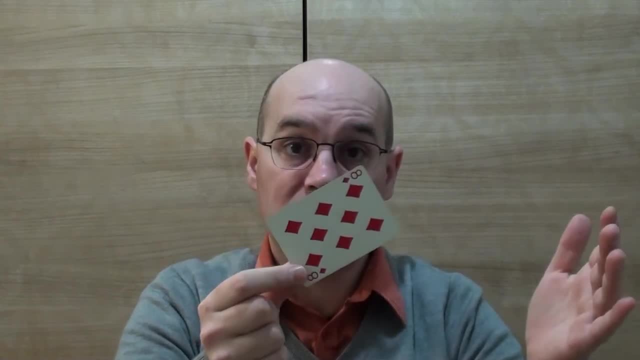 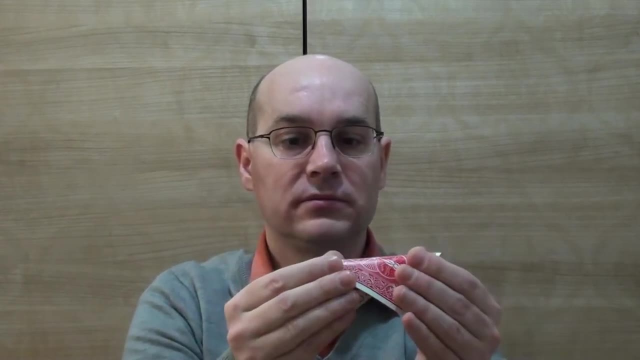 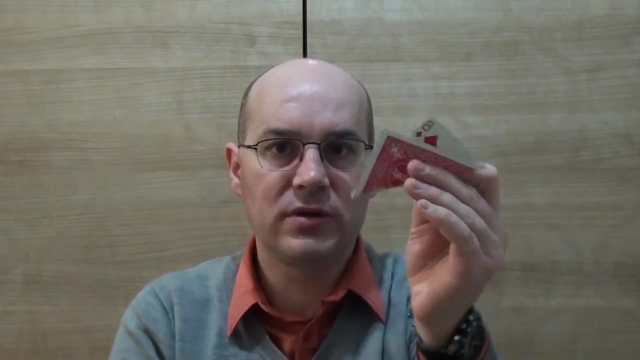 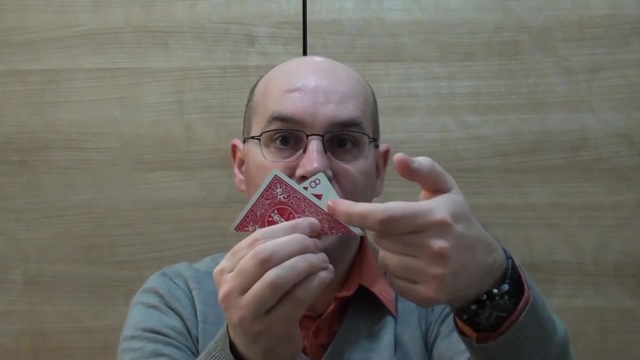 So you have two ways from this to proceed. First way is to fold along that very great diagonal like this, And you can see that you get this very strange shape. but you can see this little triangle and actually this line is where you are going to fold. 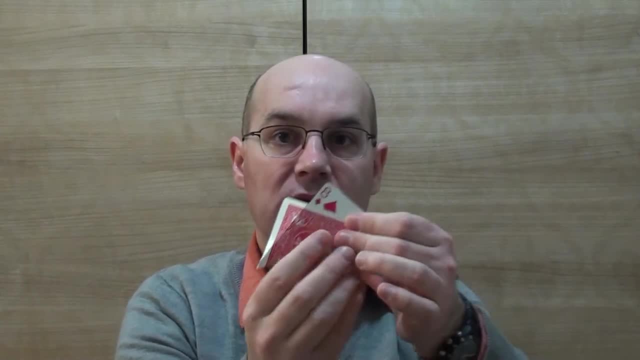 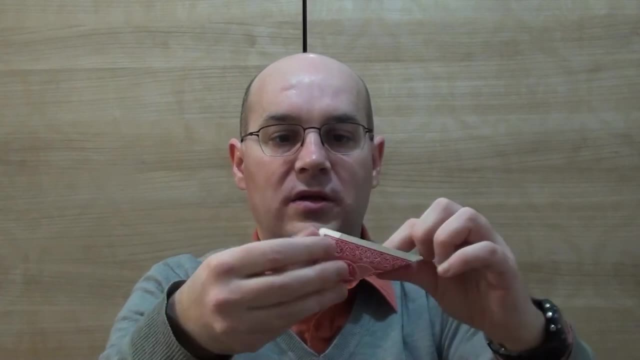 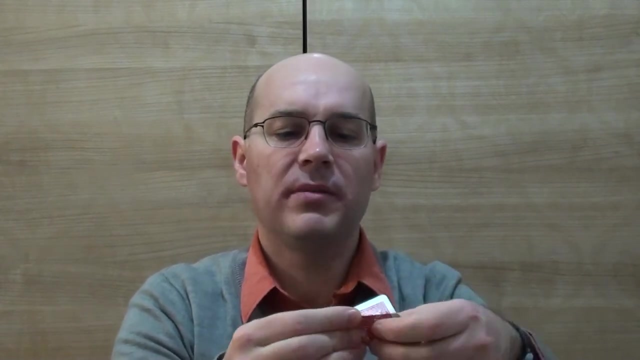 to get this rhombus And, of course, in the other way you are going to get also the other fold, which is symmetrical, And normally if you fold properly, you get something that looks a little bit better than that. It's not easy to fold playing cards. 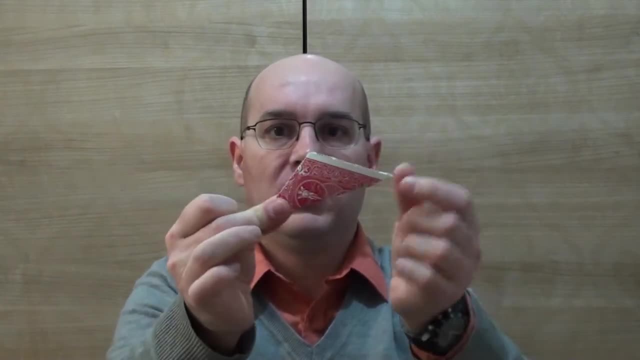 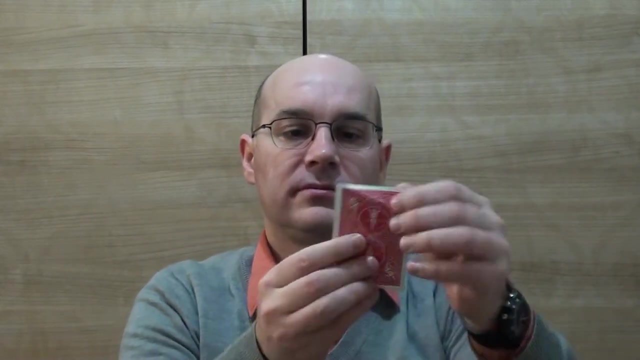 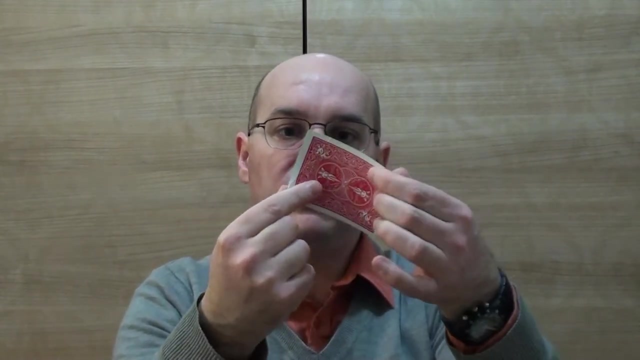 And you get something that obviously looks like a nice rhombus. Another way to do this is not to fold along the great diagonal, but, since you want to keep this diagonal, to fold from this corner to that corner, And it's especially really nice when the corners are round. 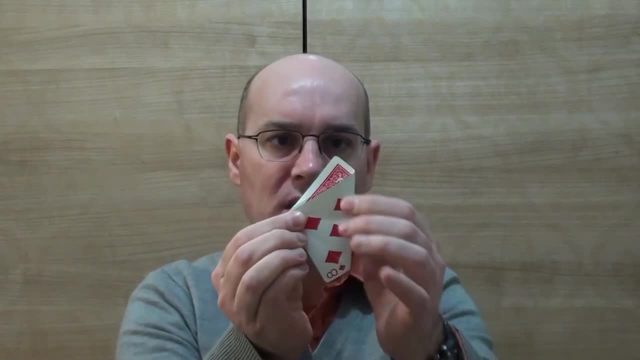 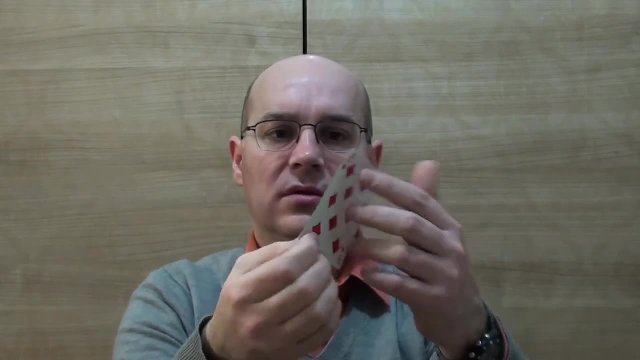 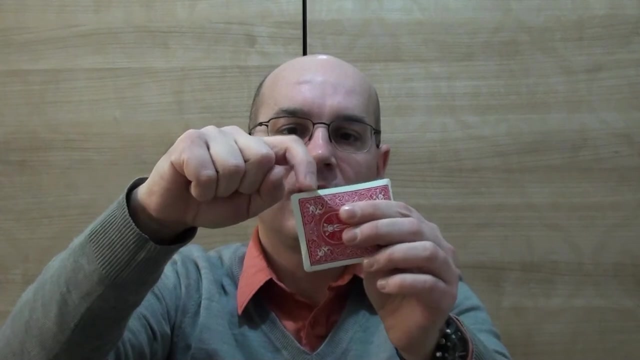 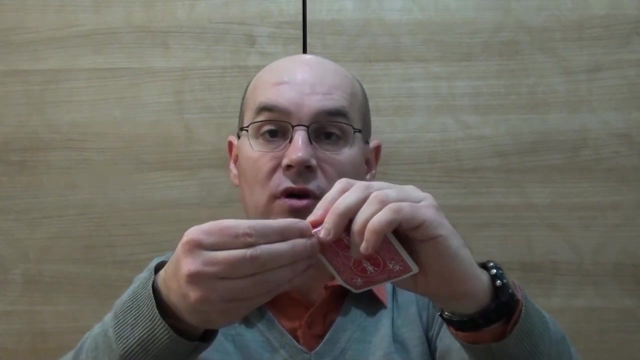 It's much easier And what you're going to get here on this, fold here. this is a small diagonal of the rhombus, So you get something like this And, of course, the small diagonal reaches just the vertex here, So you can fold here to, of course, to the corner. 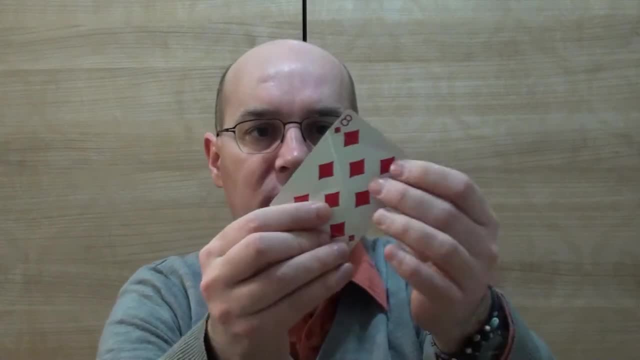 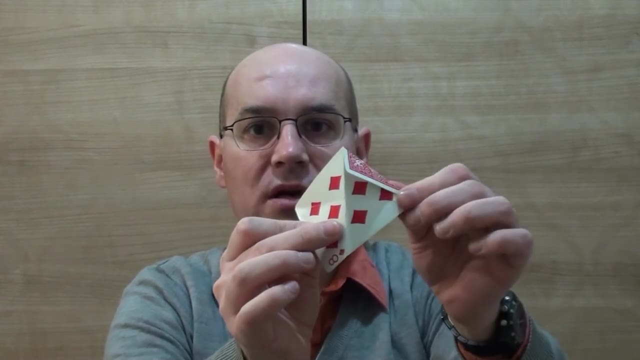 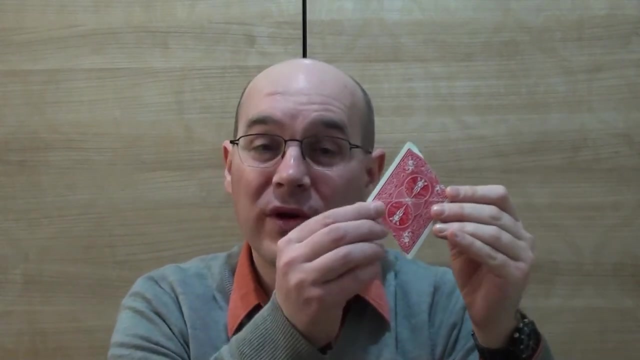 Fold here. Maybe you can see better here. So this is the small diagonal And, of course, reaches the vertex right here. So this is a second way to find the spot where to fold your playing card. Of course you're not going to fold all the cards this way.